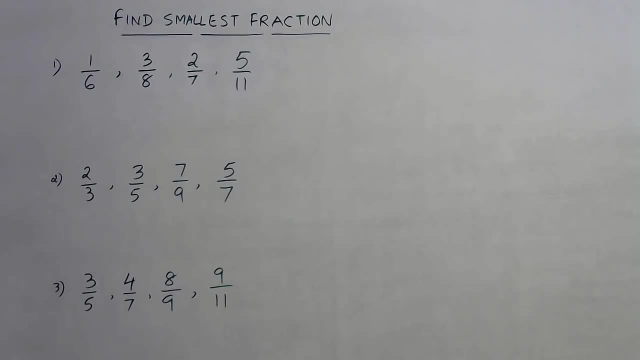 Hello friends, In my last video, I told you a method to find the largest fraction among four given fractions. In continuation to that video, I am going to tell you the shortcut for finding the smallest fraction now. Now for finding the smallest fraction. we will follow the same. 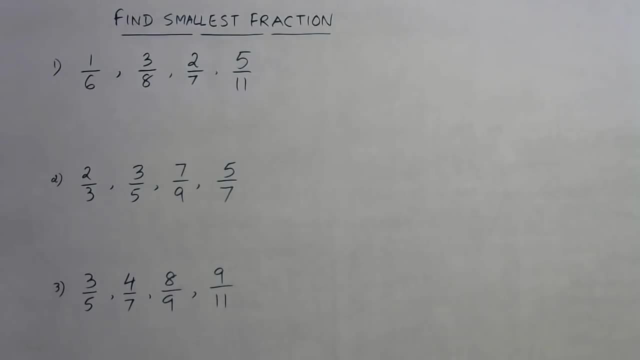 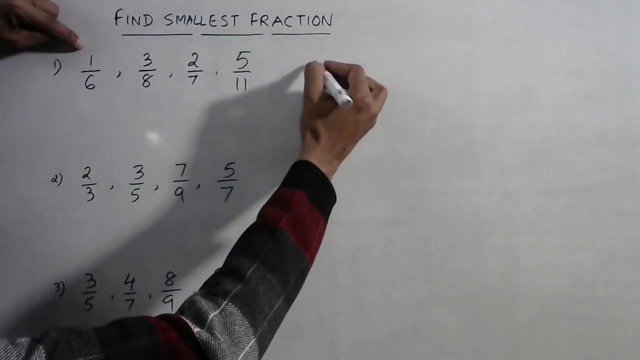 procedure which we have done in the previous video. Now let me demonstrate it in an elaborative way using the first example. Now see 1 by 6 and 3 by 8.. Take first two fractions and cross multiply the numerator of the first with the denominator of the second and numerator of the. 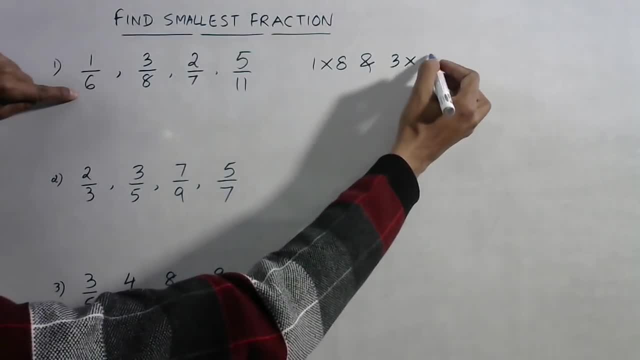 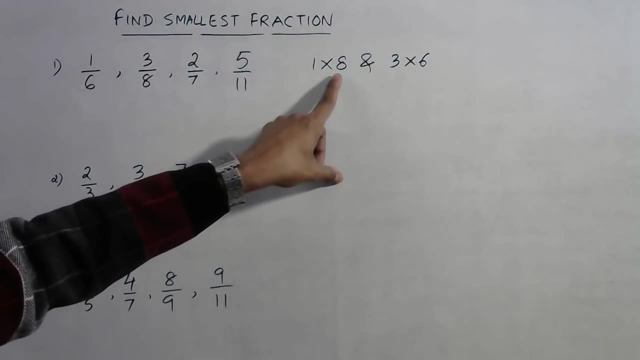 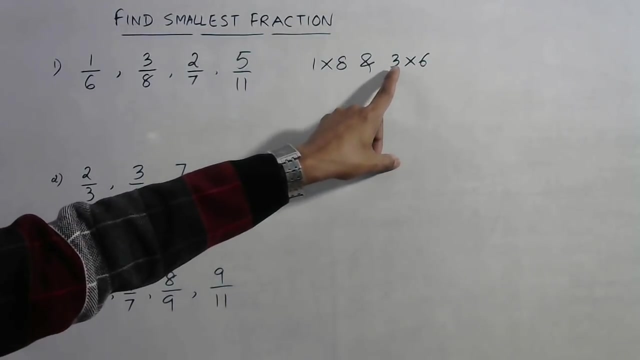 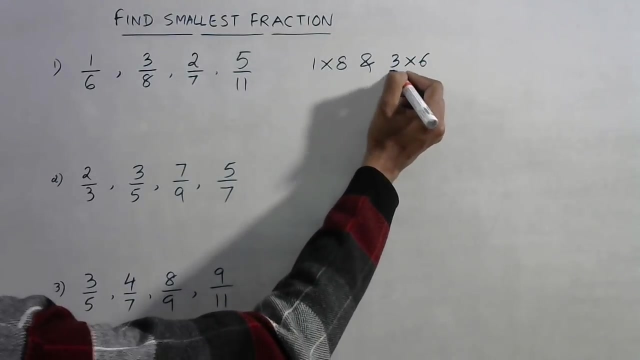 second with denominator of the first. Now we need to find the smallest fraction. So which of the two is smallest? 1 into 8 is 8,. 3 into 6 is 18.. So this is small. So we have multiplied 3 by 6. That means 3 by 8.. The numerator here is 3.. 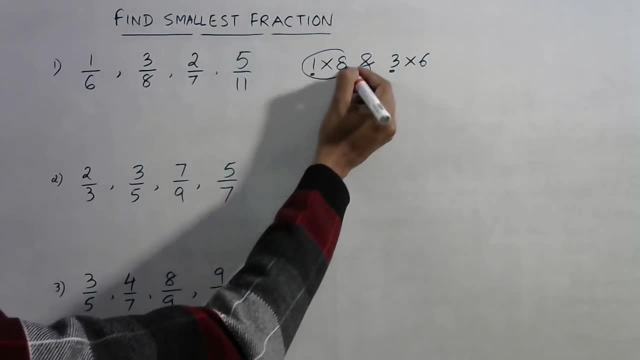 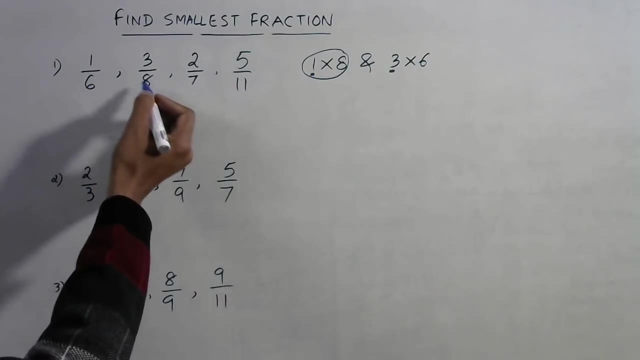 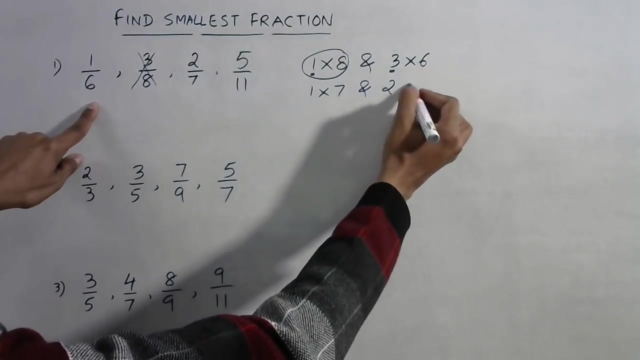 The numerator here is 1.. So this is the smaller product and the numerator here is 1.. So this is small and this is large, So we need the smallest, So discard the largest. Now compare 1 by 6 with 2 by 7.. So 1 into 7 and 2 into 6.. Now see, this product is small and this is large. 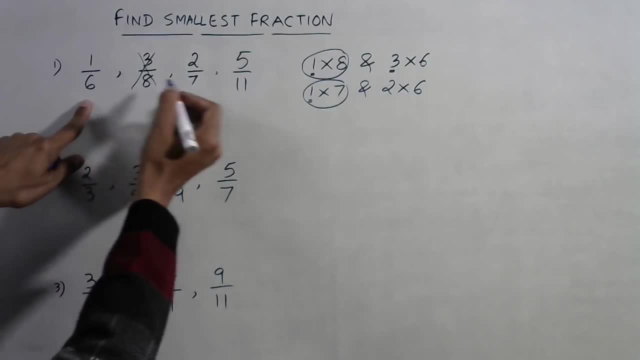 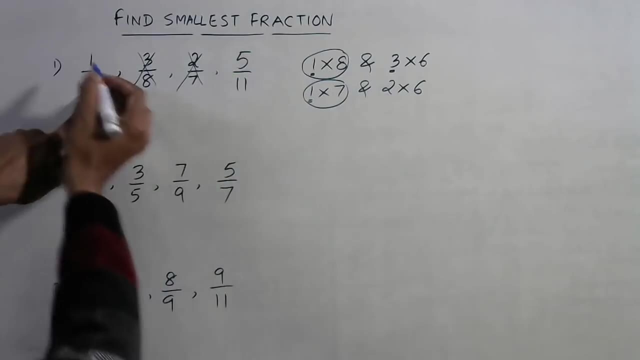 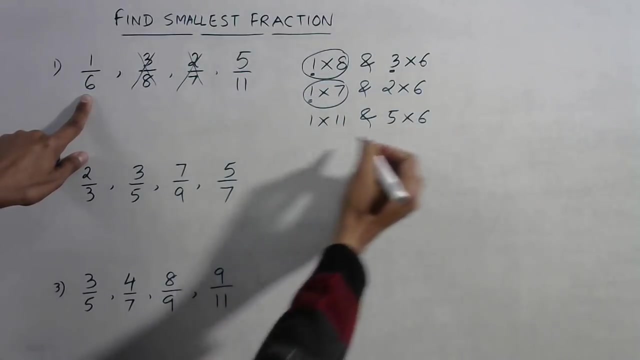 So numerator here is 1.. So 1 by 6 is small and 2 by 7 is large, So discard the larger. Now consider first and last. So 1 into 11 is 11 and 5 into 6 is 30. So which is the smallest? 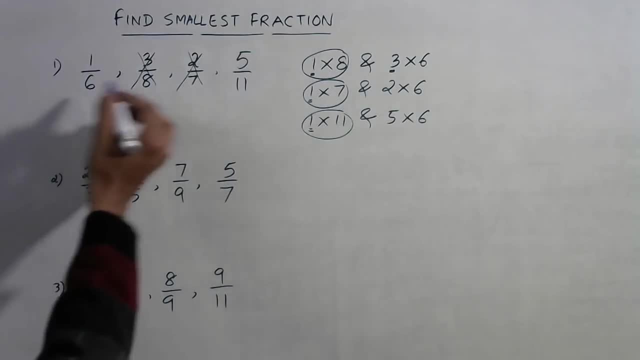 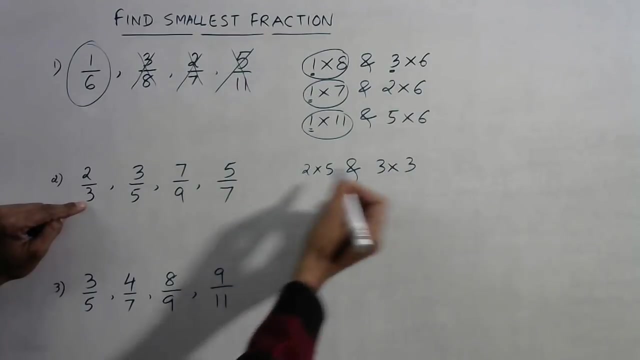 Smallest is this one and the numerator is 1.. So this is the smallest Discard. this You get the final answer, as 1 by 6 is the smallest fraction. I hope you have understood this. If not, let us take one more example: 2 into 5 is 10 and 3 into 3 is 9.. So which is small? Small is this one, and 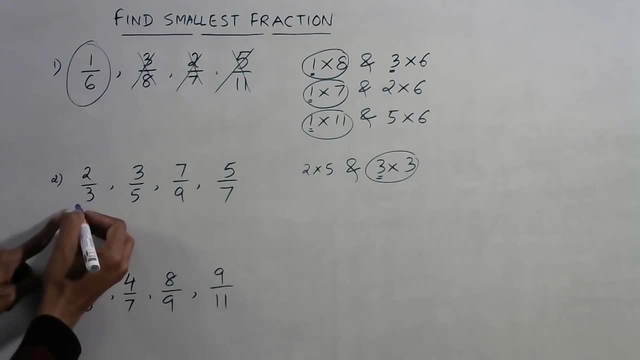 the numerator is 3.. So this is small and this is large. So this is the smallest, So this is the largest. So just neglect this. Now consider this and this 3 into 9 and 7 into 5.. Now see this is. 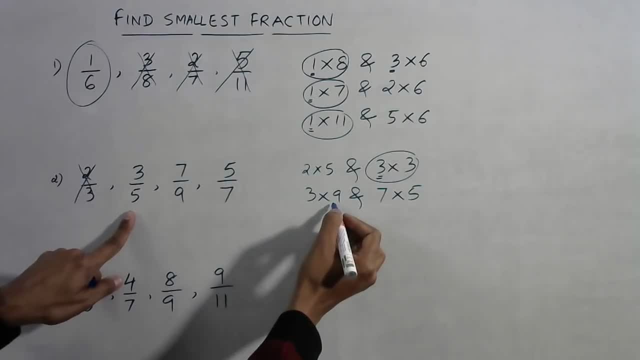 27 and this is 35. So 27 is small, So we need the small one. What is the numerator? 3.. So this is small and this is large, So discard the large one Now. 3 by 5 and 5 by 7.. 3 into 7 and 5 into 5.. 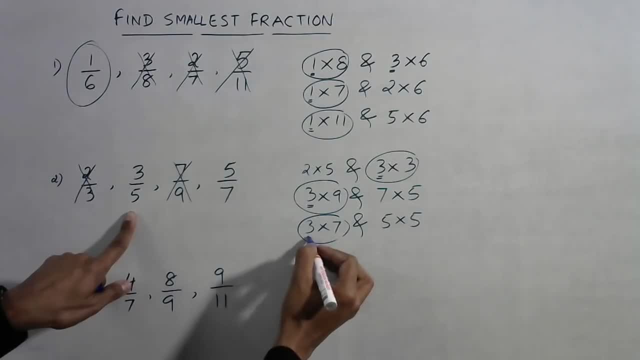 Now see, this is 21 and this is 25.. This is small and the numerator is 3.. So this is small and this is large. So discard the large, You get the smallest fraction as 3 upon 5.. Let us have the. 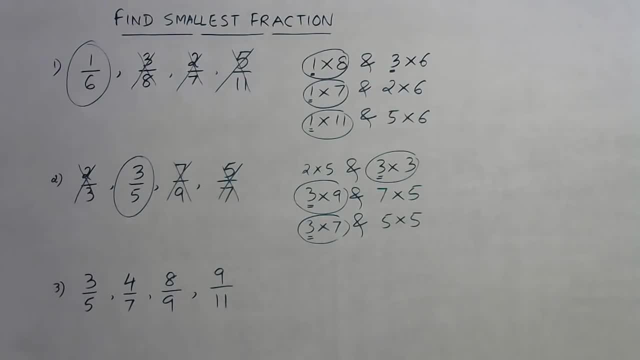 final example. Then you can practice yourself taking any 4 or 5 or even 6 fractions and finding the smallest one: 3 into 7 is 21 and 4 into 5 is 20.. So which is small of these two? 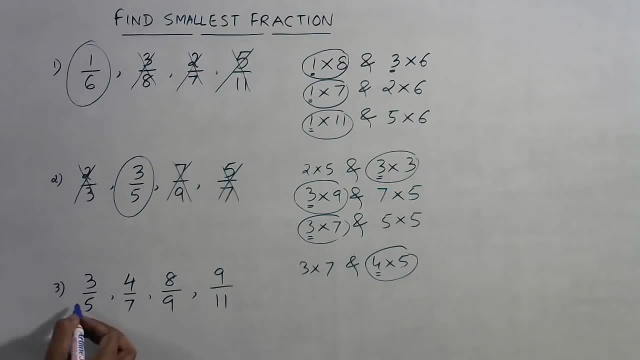 This is small and numerator is 4.. So this is smaller and this is larger. So discard 3 by 5.. Now let us have the comparison between second and third: 4 into 9 and 8 into 7.. So 8 7's are 56 and. 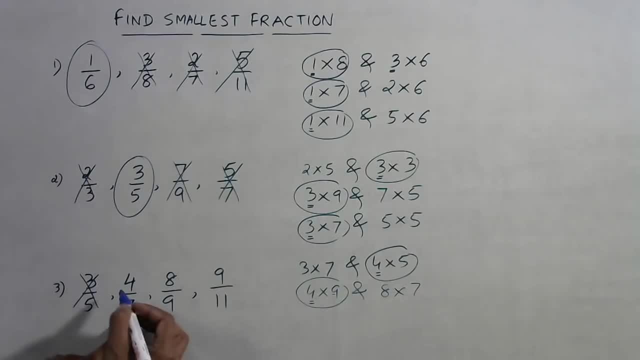 9, 4's are 36.. So this is small, So 4 is the numerator, So this is smaller and this is larger Discard, the larger. Finally, 4 into 11 and 9 into 7.. Now you see, see, this is 63. This is 44. So 44 is smaller and 4 is the numerator. 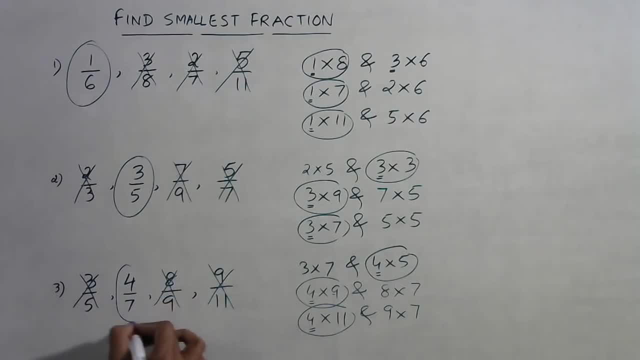 So this is small and this is large. Neglect this. You get the answer as 4 upon 7.. So, friend, this is, I think, by far the quickest method to find the smallest fraction. Practice this and I am sure you are going to save lot of time in competitive exams. For more videos, do not forget. to subscribe to my channel.